So in order to get from the vectors related to the new basis b prime to the new basis, we地 have to substitute into determinants without the ע sub u. So in order to get from the vectors using the metric permeability mode and the Porter employeesiansczę pursue the underestimating trial, we take a look at. 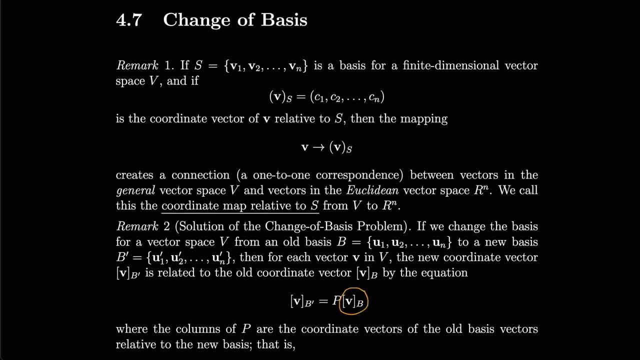 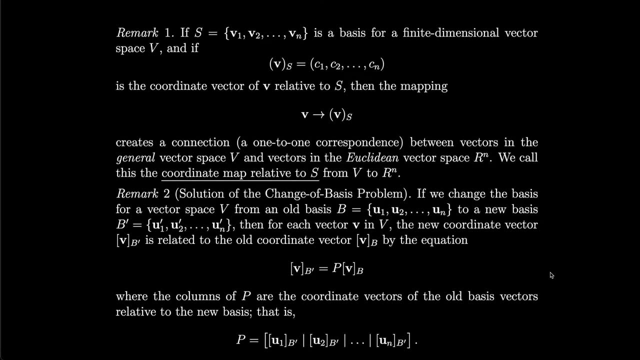 vector, the coordinate vector of v relative to b, to the coordinate vector of v relative to b, prime. what we do is we multiply by p some matrix p, where the columns of p are the coordinate vectors of the old basis, vectors relative to the new basis. so explicitly, p is equal to u1, expressed in terms: 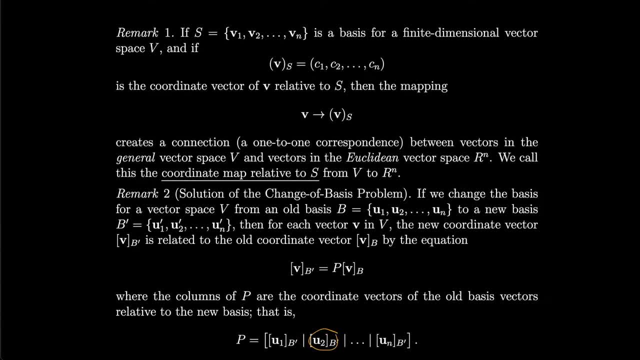 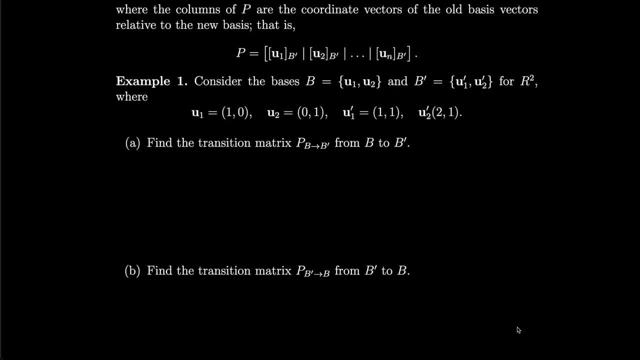 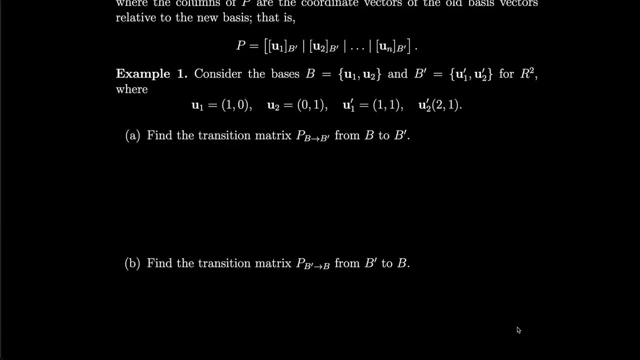 of b prime, u2 in terms of b prime through un in terms of b prime. so, as an example, how about we consider the basis: b equals u1- u2 and b prime equals u1 prime, u2 prime for r2, where u1- u2, u1. 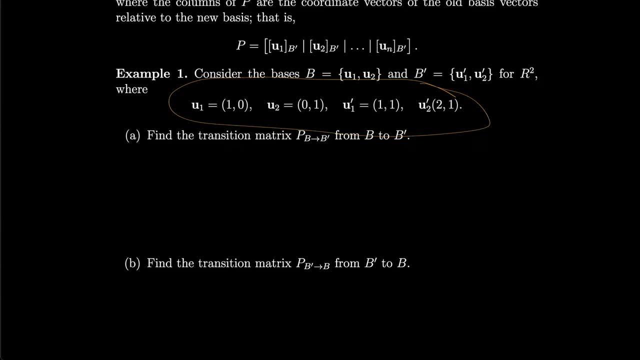 prime and u2 prime are given over here. so let's see if we could find the transition matrix p that goes from b to b prime. so we'll write u1 in terms of u1 prime and u2 prime, so it looks like u1 is 1: 0. so if i were to take 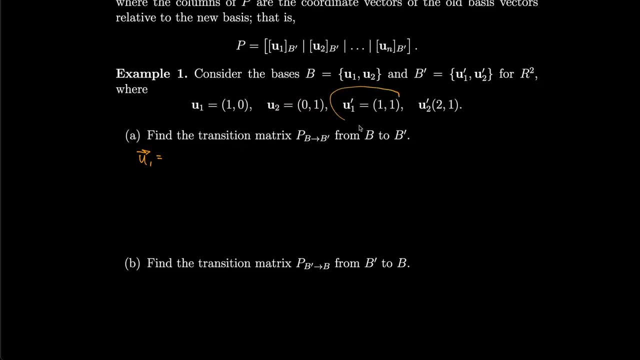 u1 prime and subtract it from u2 prime, then i get 2 minus 1 gives me the 1, and 1 minus 1 gives me the 0. so u1 must be equal to minus u1 prime plus u2 prime. we'll do the same thing for you too. we need 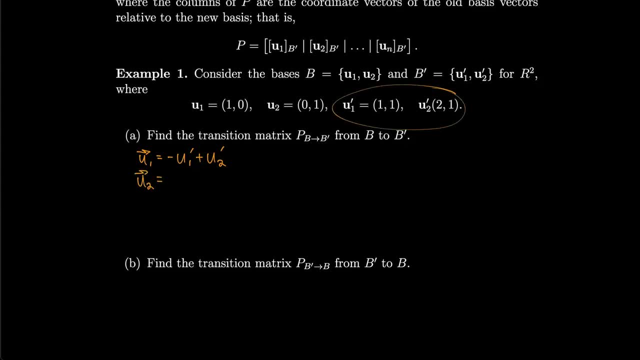 to find some combination of the primes to express u2. so what we'll do is, well, let's say u2 has zero in the first component. so how about i multiply this by 2 and then i can subtract. so i'll take 2u1 prime minus u2 prime, and yeah, that'll work, because then the 2 minus 1. 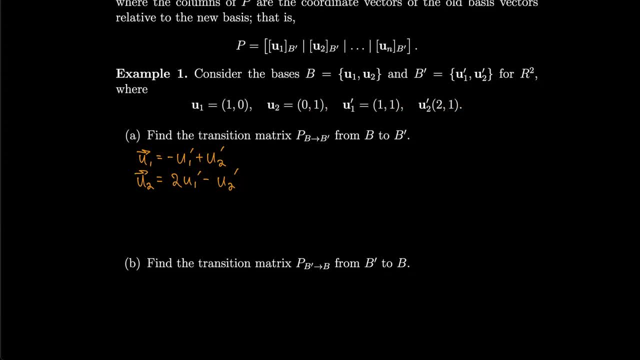 will give me a 1 there also. Okay, so now that I have u1 and u2 rewritten in terms of u1 prime and u2 prime, I can write u1 in terms of the new basis B prime as minus 1- 1, because I've got minus 1 for u1 prime and 1 for u2 prime. 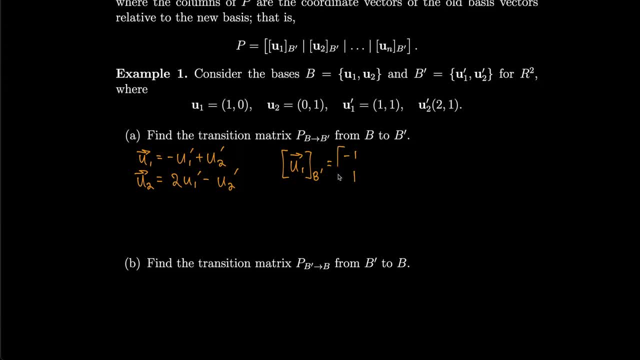 All I'm taking is the coefficients. that's what my coordinate vector will be. Do the same thing for u2.. So I want to express that in terms of B prime. now, Okay, So I already have it in terms of the primes. I just read off the coefficients and that's 2 minus 1.. 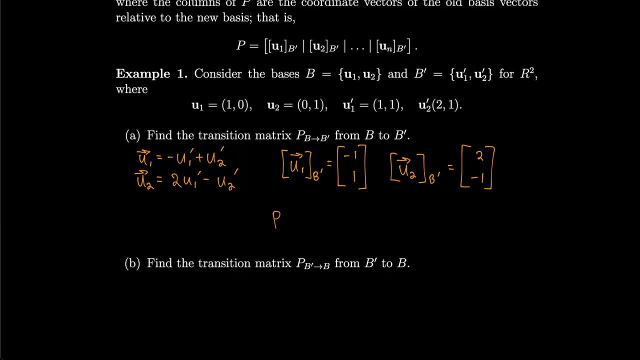 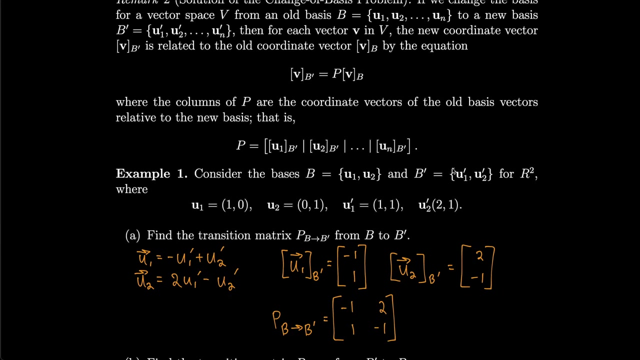 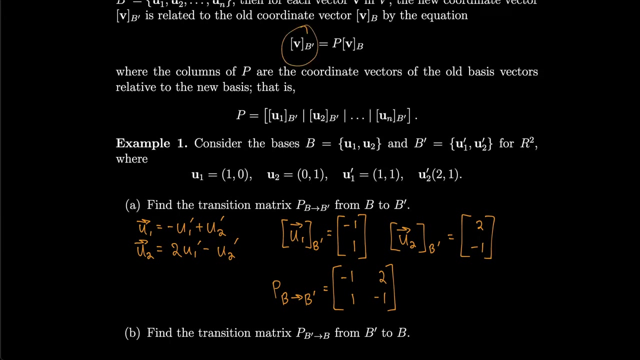 Okay, so that means that my transition matrix P that goes from B to B prime, is just equal to these column factors, so minus 1, 1, and 2 minus 1.. Okay, so if I were to take P and multiply any vector expressed in the old basis, then I would get the vector expressed in the new basis, B prime. 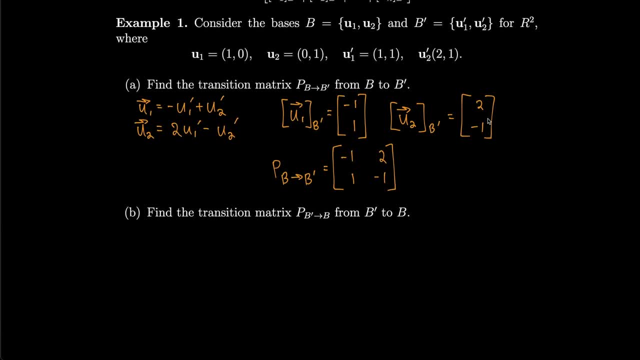 Let's do the opposite. now. How about we find the transition matrix that takes us from B prime back to B? So I need to now rewrite U1 prime in terms of the original U's, But that should be pretty easy. U1 prime is just 1, 1.. Each of these guys has a 0 in a different place, so I just need to add them together. 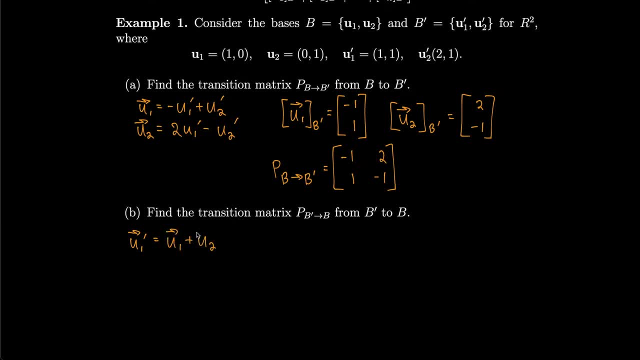 So U1 prime is just U1 plus U2.. Okay, how about U2 prime? So if I want to rewrite U2 prime in terms of U1 and U2, and there should be an equal sign over here, it's a little typo. 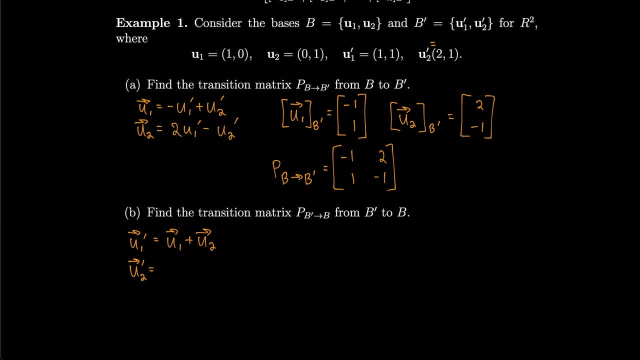 then I would take, How about 2 of U1 and add that to 1 of U2, and that gives me the 2, and that gives me the 1.. So I'll take 2U1 plus 1U2.. 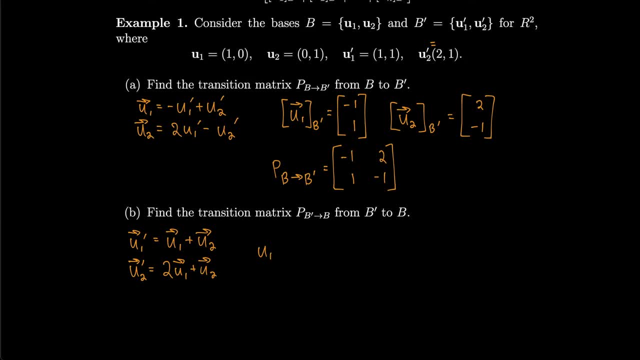 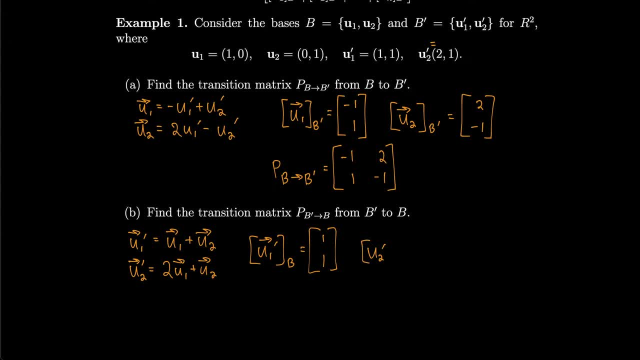 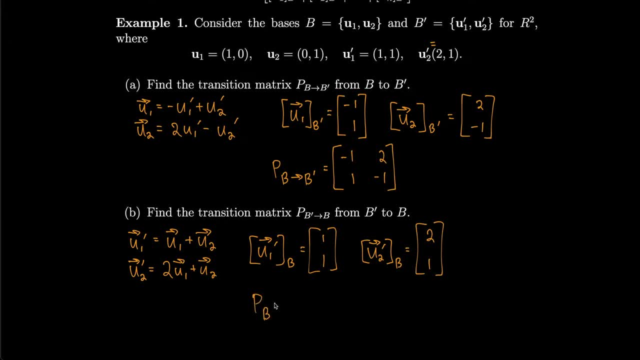 Okay, so my transition matrix from my new basis to my old one, from B prime back to B, is equal to 1, 1 and 2, 1.. 1, 1, 1. 1, 1, 1.. 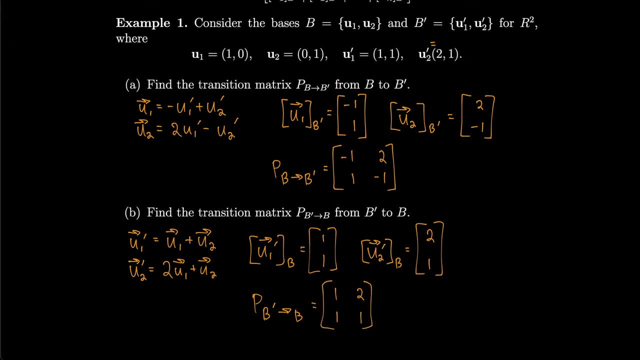 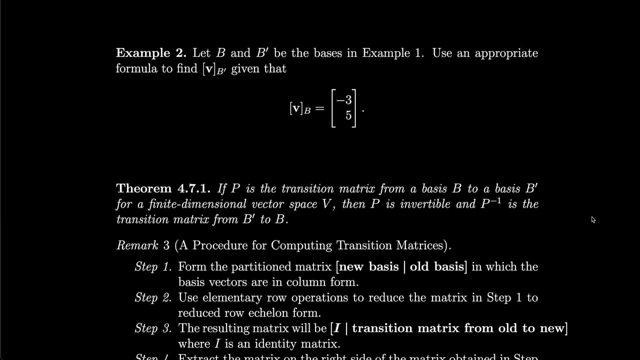 So that means that if I was starting with a vector expressed in terms of my new basis, I could get back where I started by multiplying by this transition matrix P. Okay, how about we let B and B prime be the bases in example 1.. 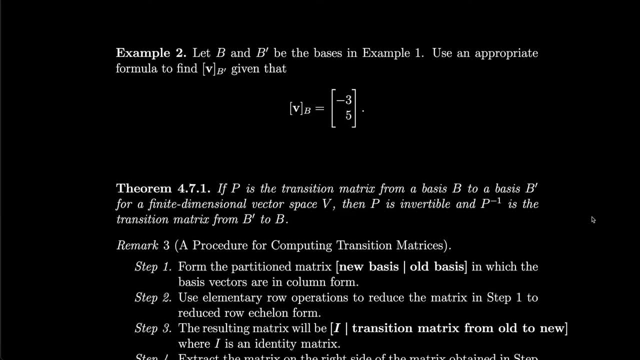 Let's use an appropriate formula to find V of B prime, given that V of B is minus 3,, 5, or VB. Okay, so I'll write VB, or I want VB prime. I'll write that as the transition matrix P, that goes from B to B prime, and I'll just multiply VB by that. 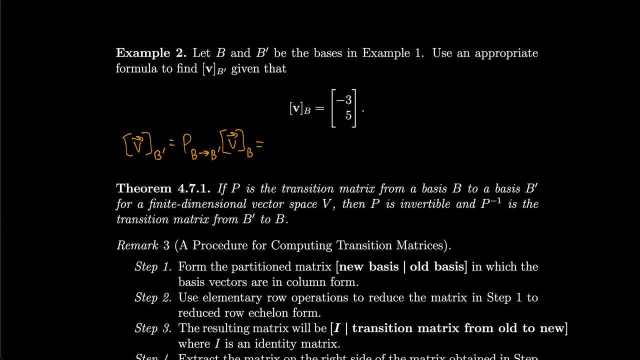 We already computed the transition matrix that goes from B to B prime. That's minus 1, 1.. 2, minus 1.. So we'll multiply that by minus 3, 5.. And we just get 13 minus 8.. 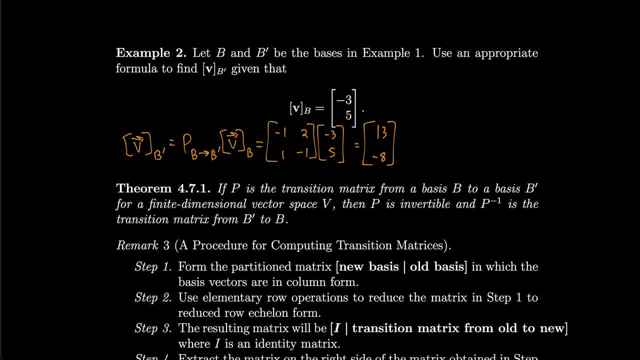 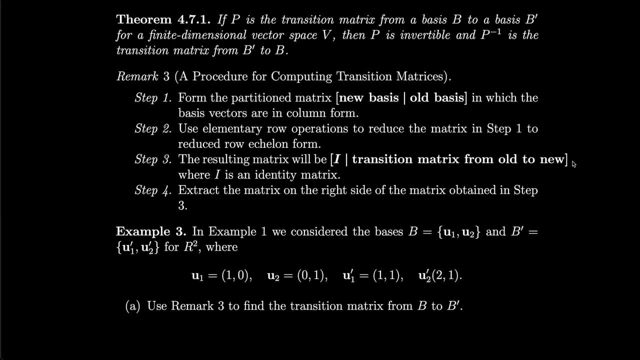 So that's the vector expressed in terms of the new basis vectors B prime. If P is the transition matrix from a basis B to a basis B prime for a finite dimension, vector space V, then P is invertible and P inverse is the transition matrix from B prime to B. 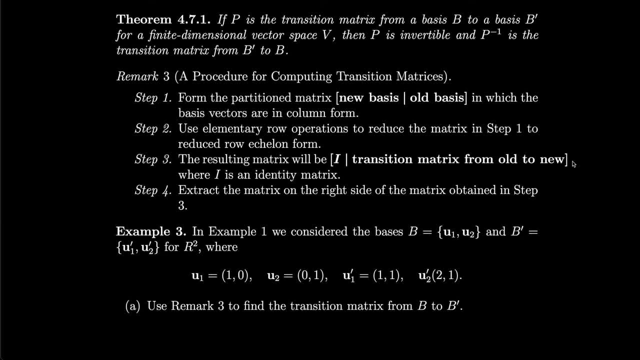 We have a procedure for computing transition matrices. What we can do is form the partition matrix where the left part of the matrix is the new basis and the right part is the old basis, in which the basis vectors are in column form. Then we can use elementary row operations to reduce the matrix in step 1 to the reduced row echelon form. 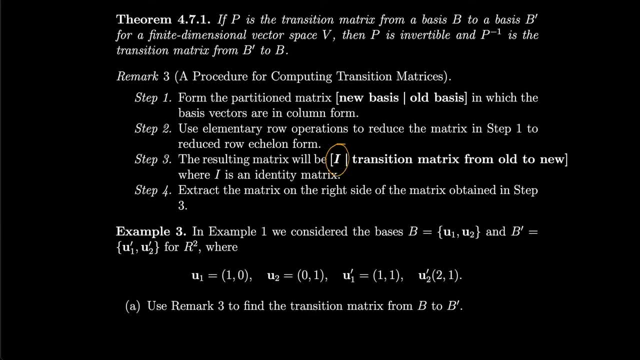 and then set up a new matrix. The resulting matrix will have the identity matrix in the left and it will be adjoined to the transition matrix from old to new. So this is exactly what we want, And that's it. We get it. 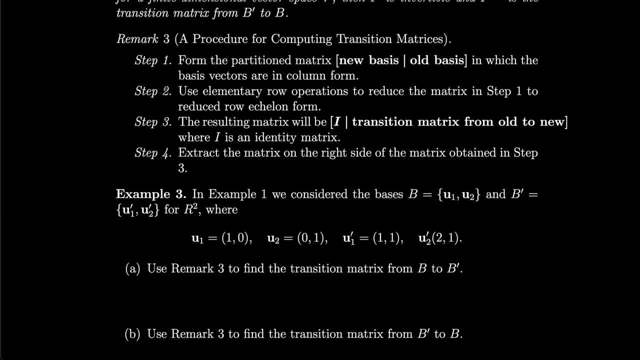 As an example, how about we consider the basis B and B prime before Let's use this new procedure to find the transition matrix from B to B prime? So what we'll do is we will form a new matrix consistent with this new matrix. 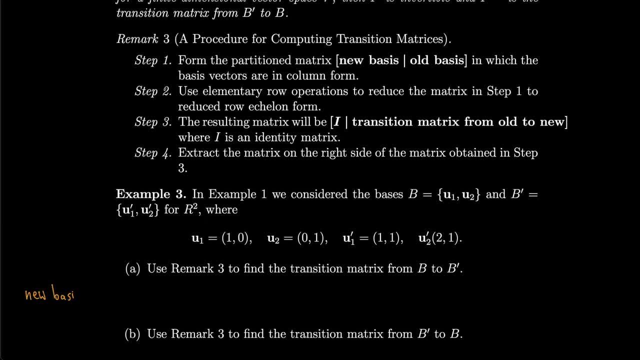 So what we'll do is we will form a new matrix consistent with this new matrix of the new basis adjoined to the old basis, and we'll set that equal to 1, 2 1 1. that was my old basis for the vectors. actually, I want to just adjoin that to. 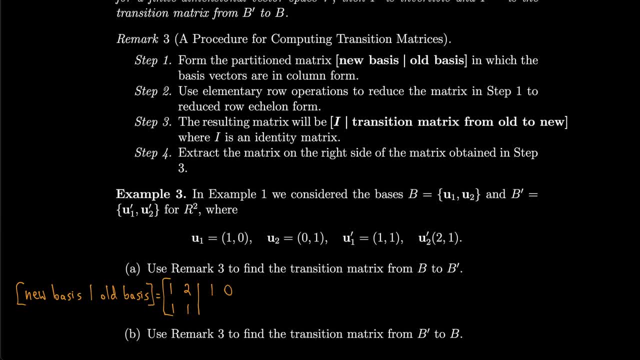 it was a 1 0 0 1, it was the standard basis. okay, so then I'm going to reduce that to the identity in the left, and on the right will be my new transition matrix from old to now. okay, so I can subtract off over here to get this to become the identity I'll. 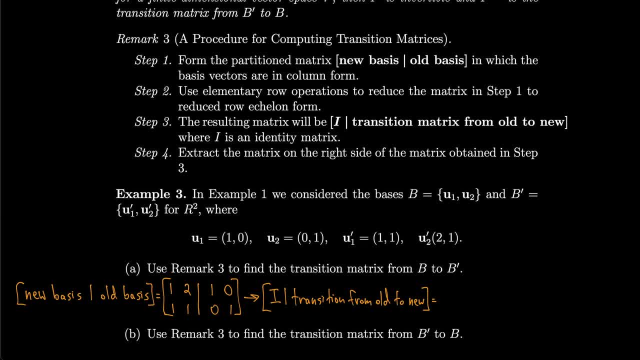 subtract off 2 of this and then make it negative, because if I subtract off 2 then this becomes a minus 1. make it negative, become positive. so I'll get 1- 0 and I'll get minus 1- 2 and in the bottom I just need to subtract off 1 of those to cancel out. 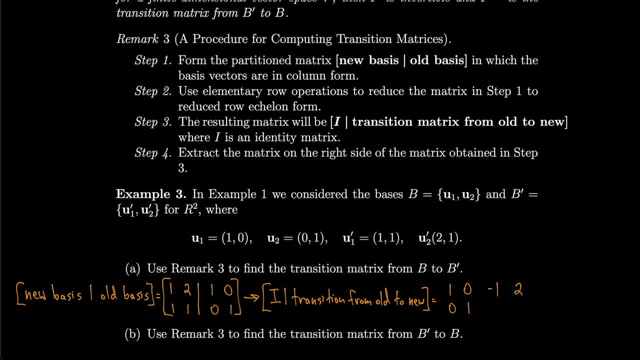 that 1 and get 0. so I'll just get 0, 1 and 1 minus 1. okay, so there we go. that means that my transition matrix is incomplete. now very small zwischen� and 1 d 1. my transition matrix is on the right, so that's b to b prime and, as before, it is equal to minus one. 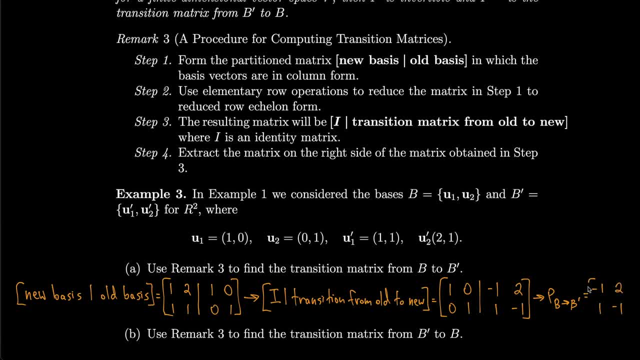 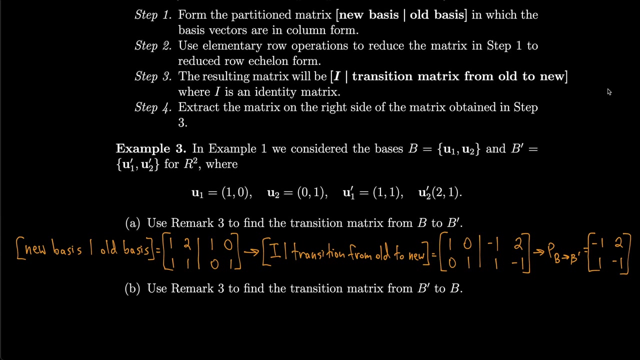 one, two minus one. so this gives us an alternative way of computing it, in kind of like a brute force way, instead of having to find some way to rewrite our basis vectors in terms of the other basis vectors. okay, how about we do the same thing from b, prime to b, so i've got my new basis. 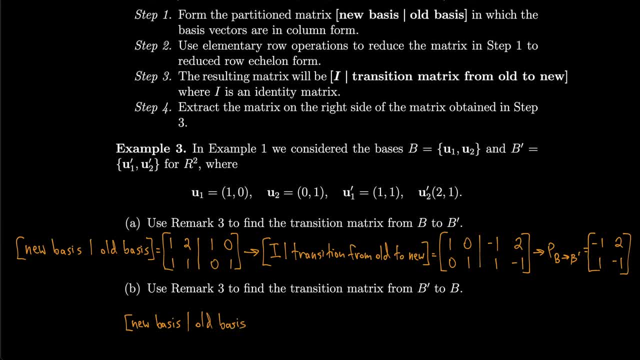 my old basis and my new basis. in this case i'm going to b, so that's my new basis. so that's just the one, zero, zero, one basis, and my old one is one, two, one, one. but notice, this is very easy to solve because this is already. 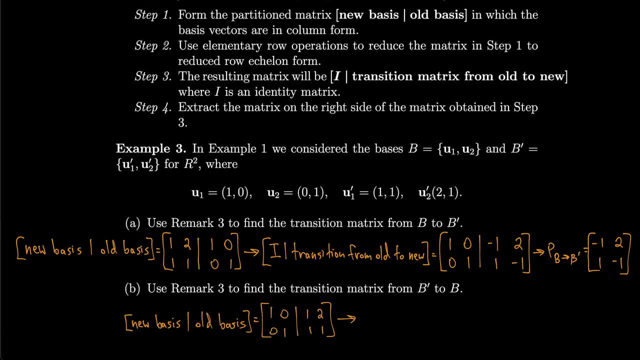 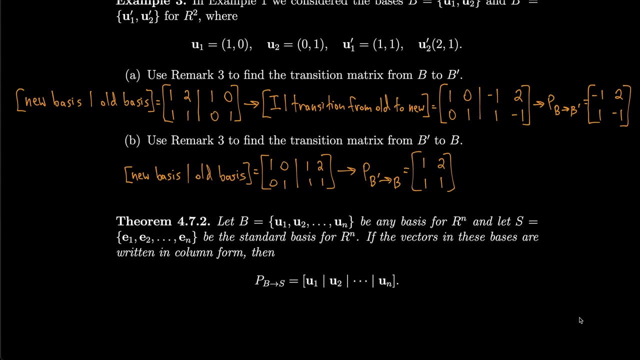 reduced. so that means that my transition matrix to go backwards is literally just the new basis or the matrix formed by the new basis. so that's p from b, prime to b, given by one, one, two, one again matches what we got before. let b equal u, one through u, n be any basis for rn and let s equal e1 to e- n be the standard basis. 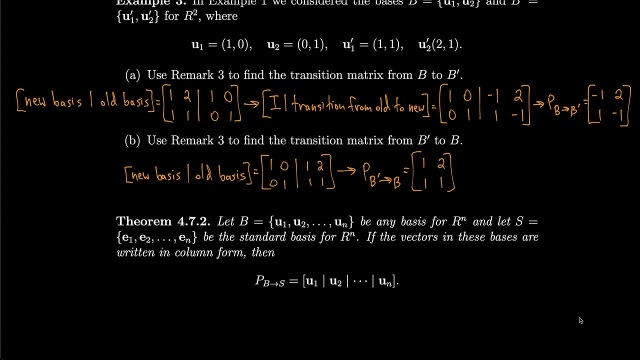 for rn. if the vectors in these bases are written in column form, then the transition matrix from b to s is just the basis vectors. the new ones basically follows pretty clearly from the remark that we just did. obviously it's not a proof, but it should be a little bit more convincing now. 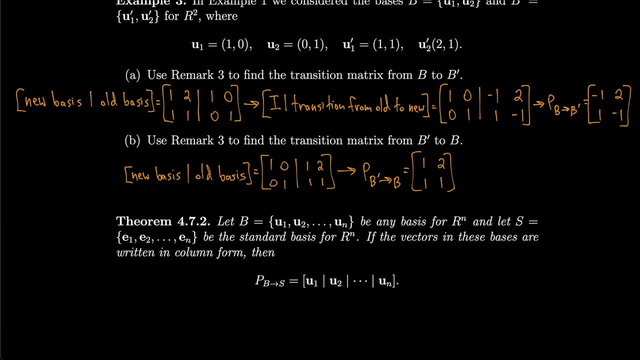 that this is true, given we just saw the previous session. so we've done that now. so we're just going to compute the new basis vectors and then we'll do the same thing to the old basis matrix. so that's. We saw this in the last example.